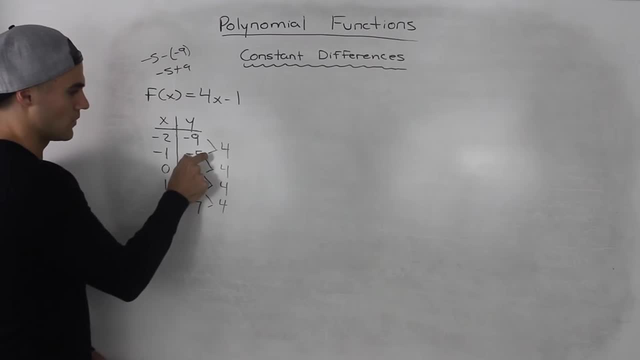 times throughout this video, because it's a common mistake. you always take the bottom y value. subtract the top y value. Bottom y value: subtract the top y value. Bottom y value: subtract the top y value. A lot of students what they do is they take y values. 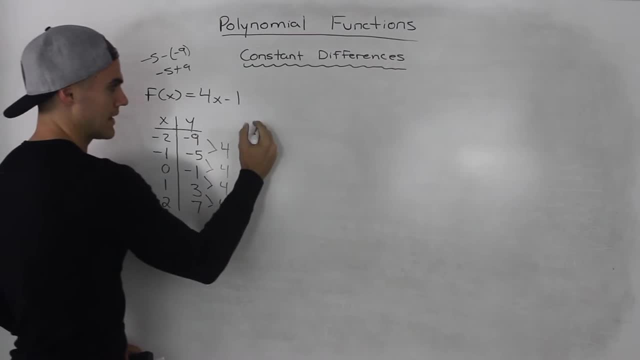 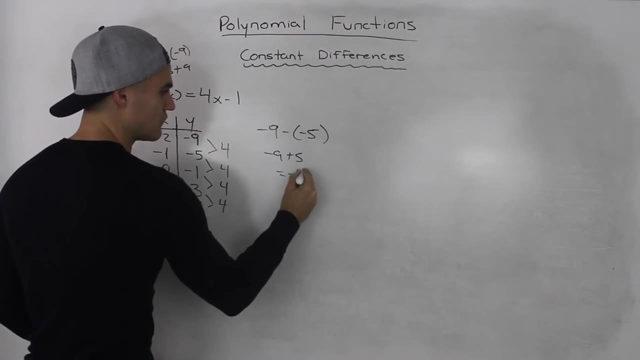 the bottom y value and subtract the bottom y value, which would be wrong, because if we took negative 9 and subtracted negative 5 from it, that would be negative 9 plus 5, which would give us negative 4, and that would be a different answer. So make sure that you're. 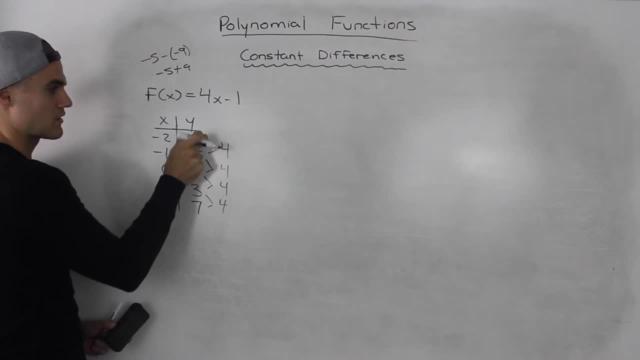 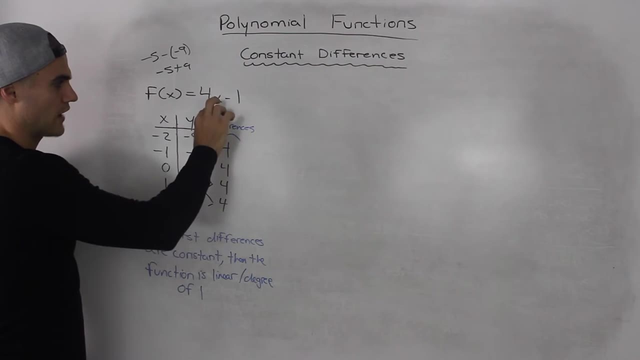 always taking a y value and subtracting the top y value from it to get your differences. Now, this column of 4s here are called our first differences because it's the first column that we made. We're subtracting this table of values And notice how this column is constant. It has. 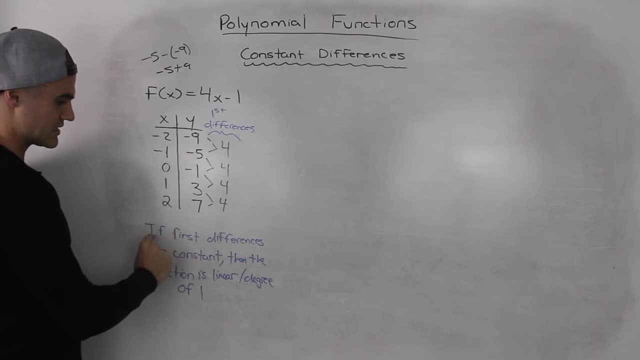 a constant value of 4.. So since the first differences are constant, then the function that we're dealing with, we know, is linear or has a degree of 1.. So in this case we already knew we were dealing with a linear function, because we were given 4x minus 1, which has 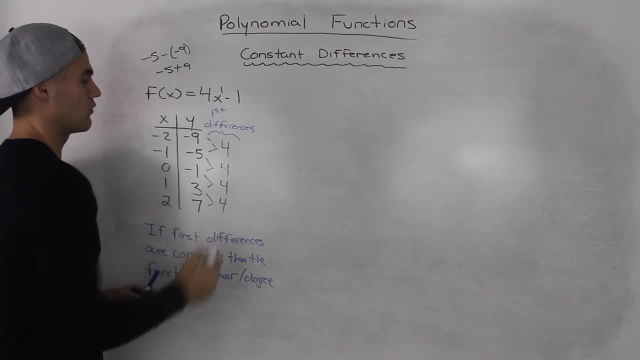 a degree of 1, x to the power of 1 there. However, if we were just given this table of values and we weren't given this function algebraically and we took the differences because the first differences were constant, we know that this function would have been linear. So it's a nice way to check what degree. 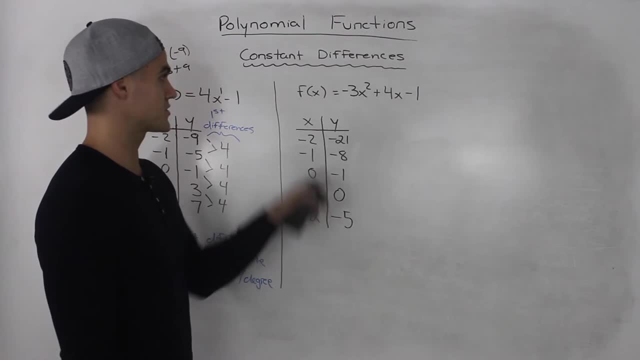 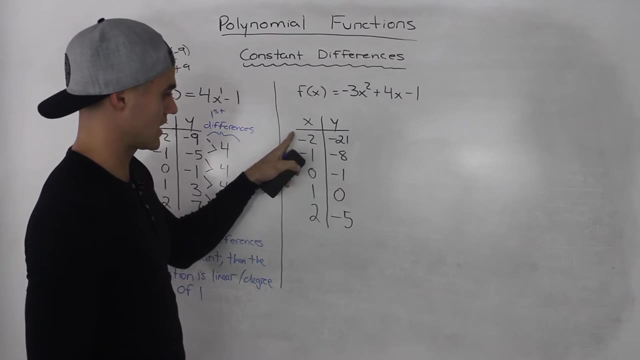 of function you're working with, Moving on to the next example. so f of x equals negative 3x squared plus 4x minus 1.. I made a table of values for it, from x values, negative, 2 to positive 2.. So now that we have our table, 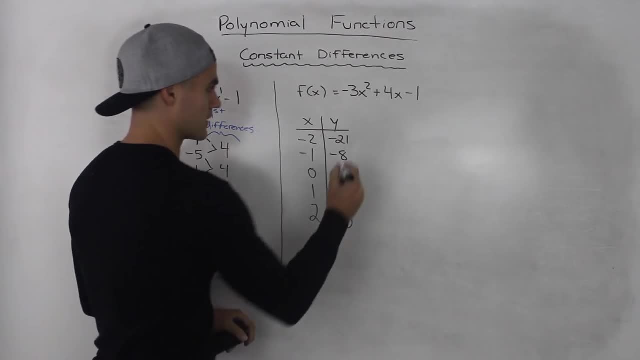 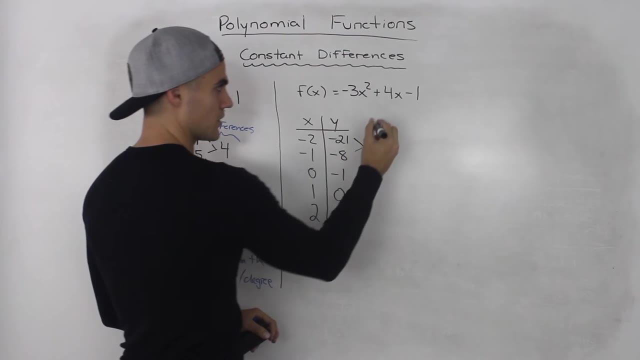 of values. let's make sure that we have our table of values. Let's make sure that we have our table of values. Let's find what the first differences would be. So what do we do? We take this y value and subtract the top y value, So negative, 8 minus negative. 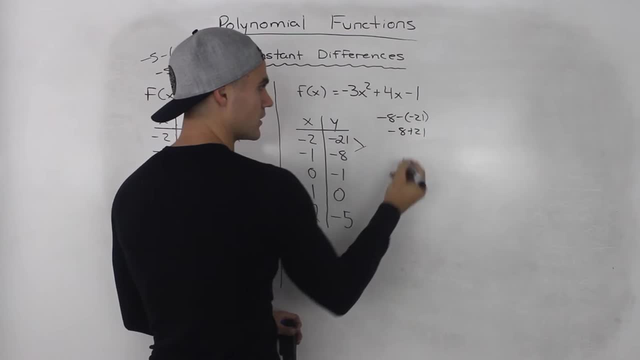 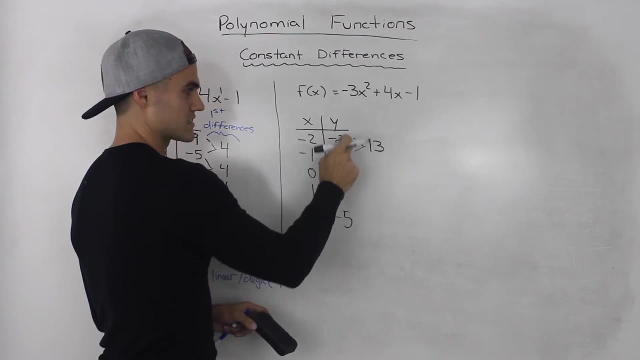 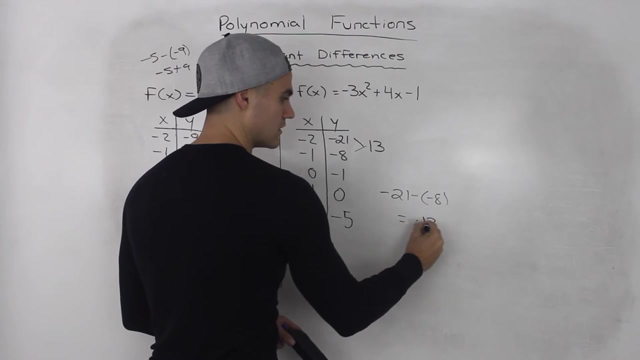 21 would be the same as negative 8 plus 21,, which would give us 13.. Notice again how we took the negative 8 and subtracted negative 21.. We didn't take negative 21 and subtracted negative 8 because that would give us negative 13.. 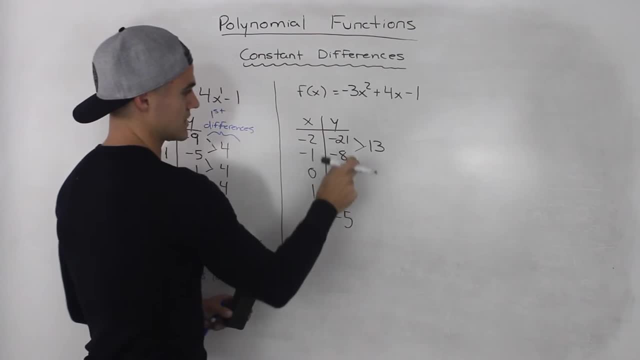 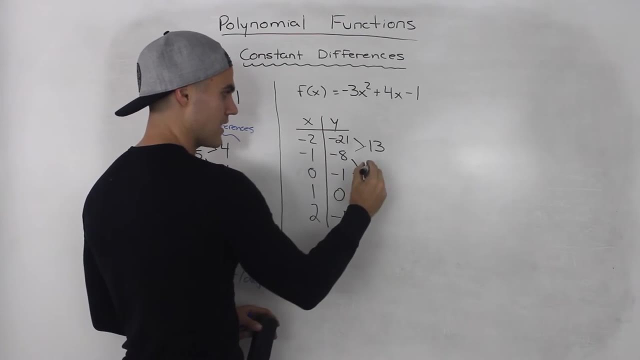 And that would be incorrect. Right, So you always take the bottom y value and subtract the top y value. So let's move on to the next one. Negative 1 minus negative 8 would give us positive 7.. 0 minus negative 1 would give us positive 1.. Negative 5 minus 0 would give. 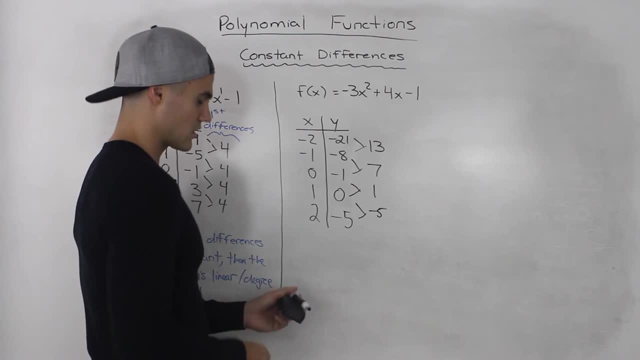 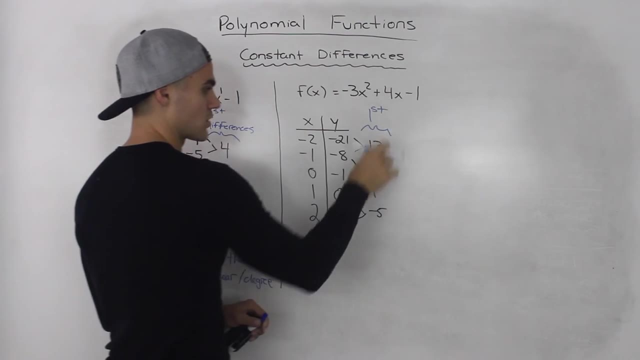 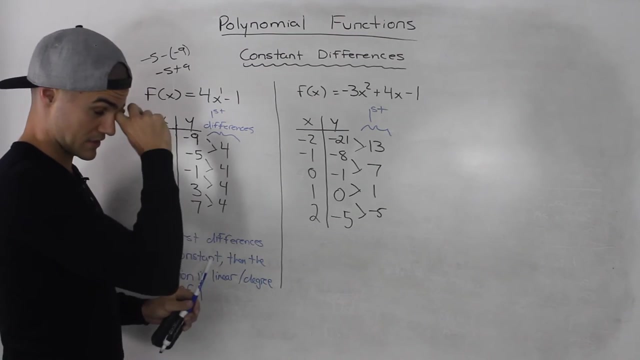 us negative 5.. So this column right here is our first differences. I'm just going to put first here These are our first differences And notice here how they're not constant as they were in this example. So if the differences aren't constant, what we have to do is we have to take the 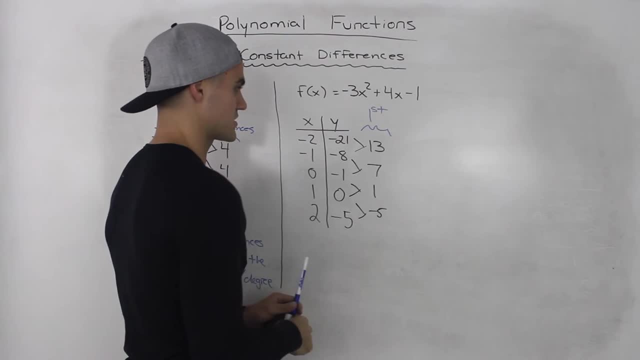 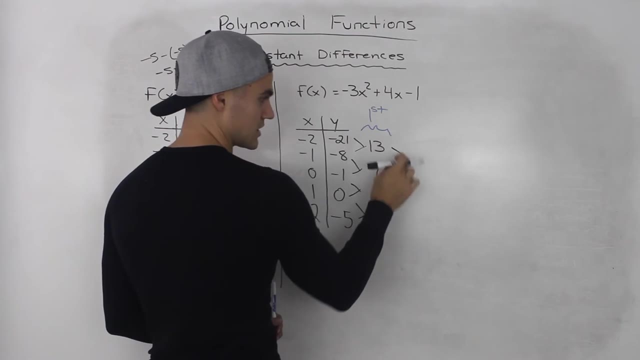 differences of this column now and find our second differences. And the same thing applies. We take the bottom value and subtract the top value. So 7 minus 13 would give us negative 6.. 1 minus 7 would give us negative 6.. Negative 5 minus 1 would give us negative 6.. And then 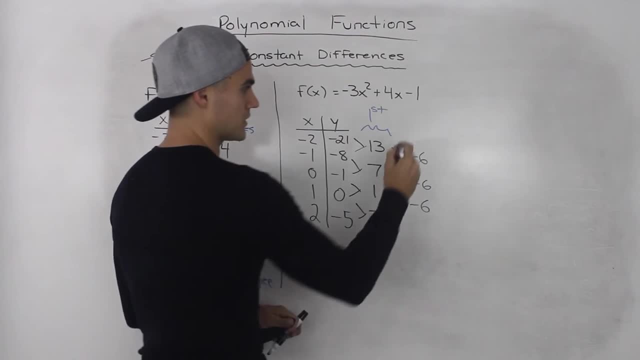 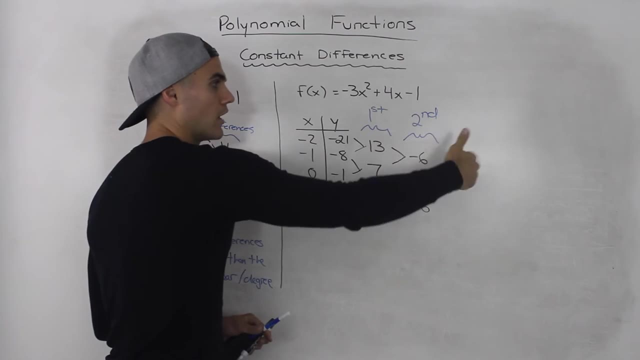 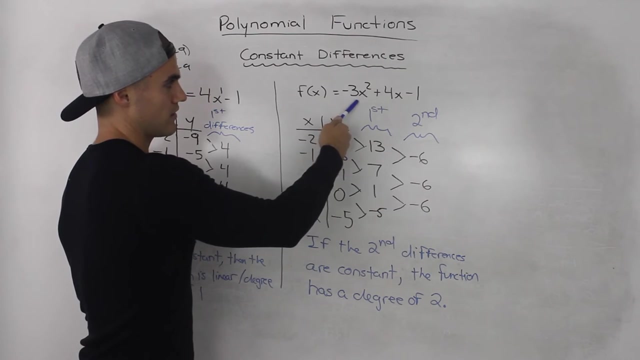 we subtract the top value, So 7 minus 7 would give us negative 6.. And this column here is our second differences. And we could keep going on and on and find our third differences, fourth differences, etc. etc. So the second differences were constant and we're dealing with a function with a degree. 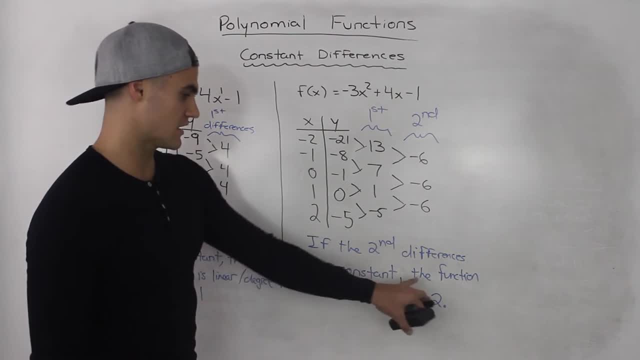 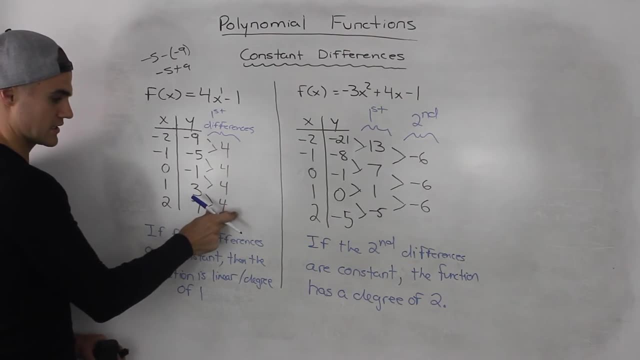 of 2.. So if the second differences are constant, then the function has a degree of 2.. And are you noticing a pattern here? So the first differences were constant. here We subtract the top value and subtract the bottom value. That means that the first differences 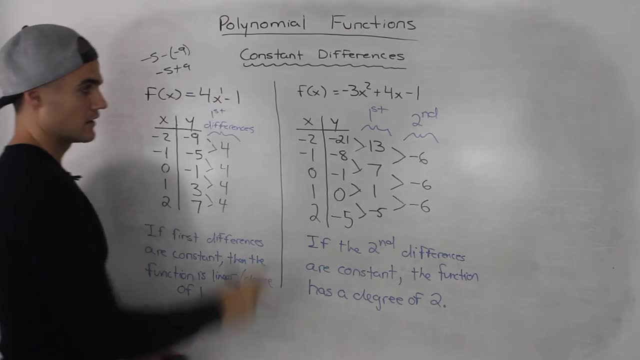 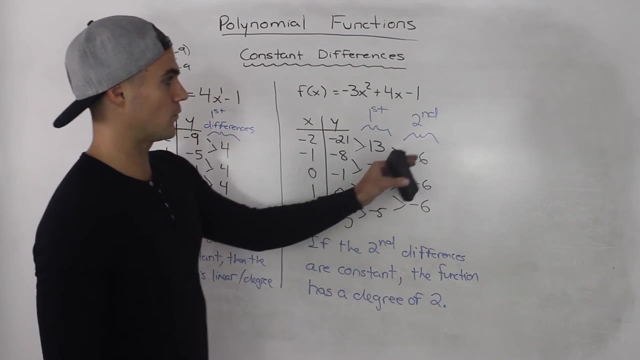 and this function was a degree of 1.. Second, differences were constant here, and this function is a degree of 2.. So it seems like that whichever column first, second, third and so on and so on, whichever column has the constant. 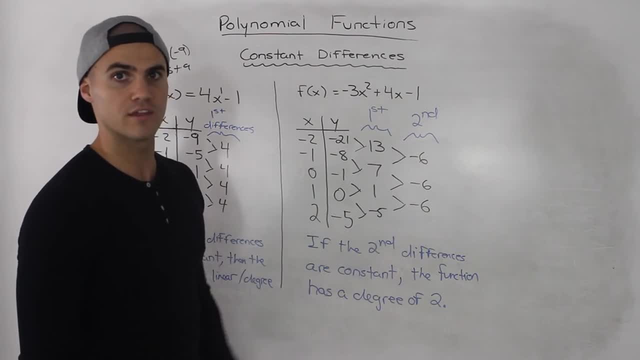 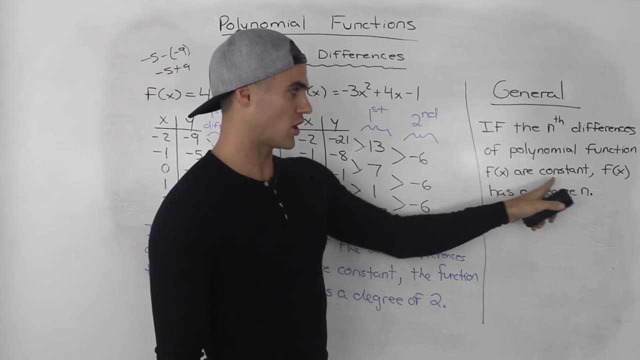 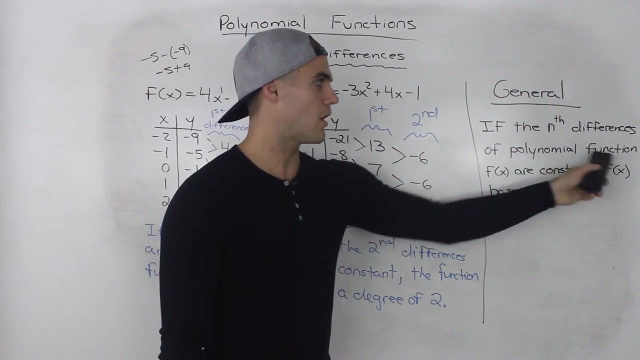 differences, that is the degree of the function. So the general observation is: if the nth differences of polynomial function f of x are constant, that means f of x has a degree n. Another thing to keep in mind is that we're still dealing with polynomial functions. for this section, Constant differences only apply. 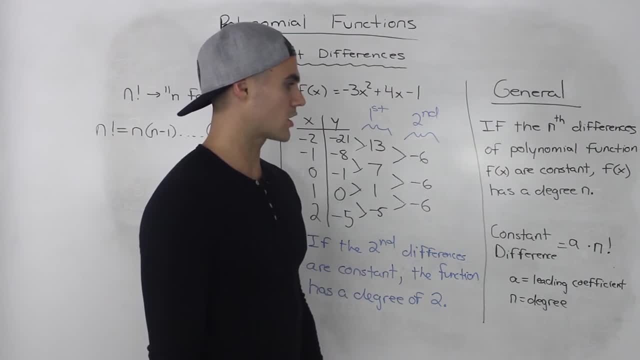 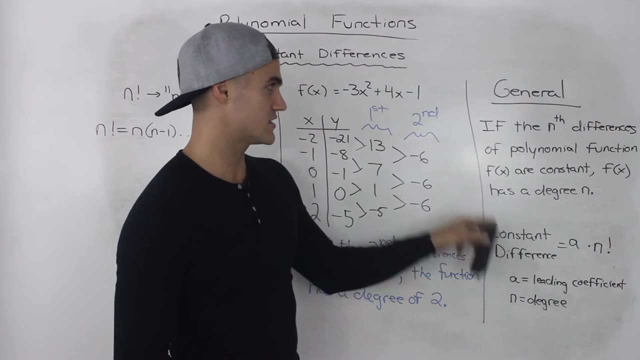 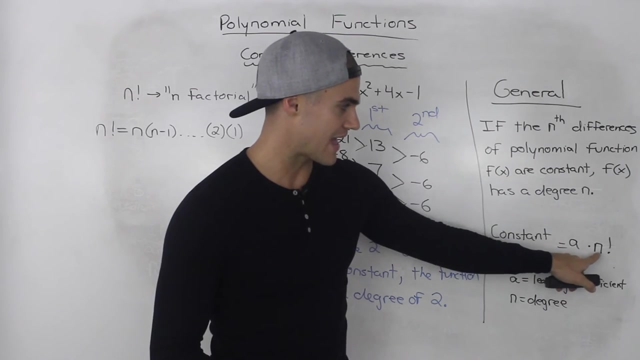 to polynomial functions. Now, the last thing I want to talk about before finishing up this constant difference overview video, is that there's an actual way to find the constant difference if you're given an equation and that's just equal to a, which is the leading coefficient times n, factorial or n. 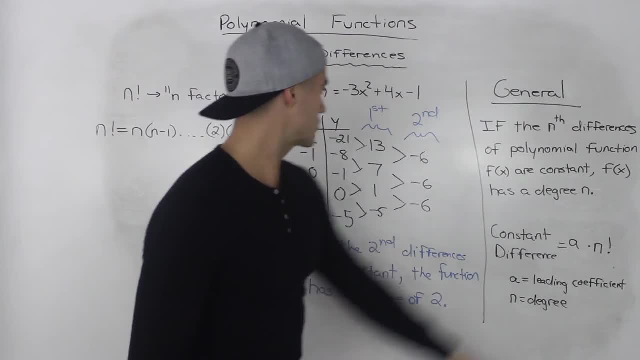 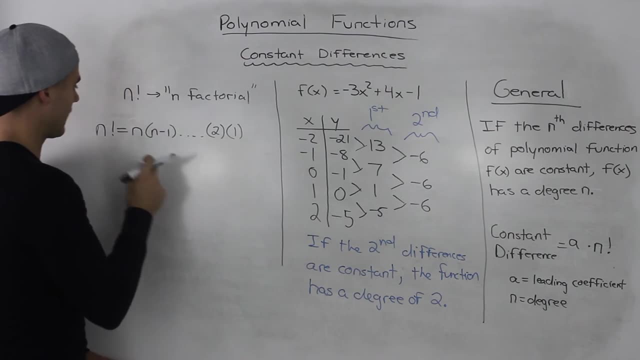 degrees This exclamation mark. So let's go over what that means. So this n exclamation mark the way to say that is n factorial, And all that means is that you take your n value and you multiply it by all the numbers below it, all the way up to 1.. So 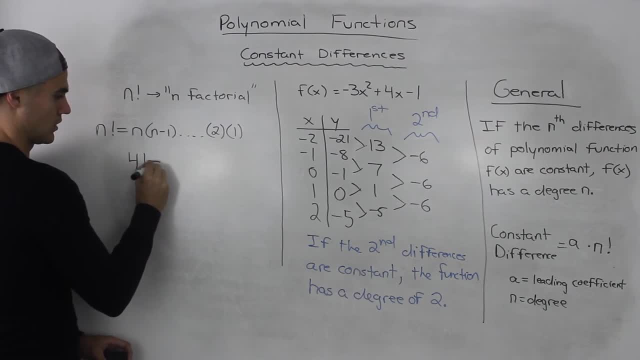 for example, 4 factorial would be equal to 4 times 3 times 2 times 1.. We always end at the 1.. So 4 times 3 times 2 times 1 is equal to 24.. So 4 factorial is equal to 24.. 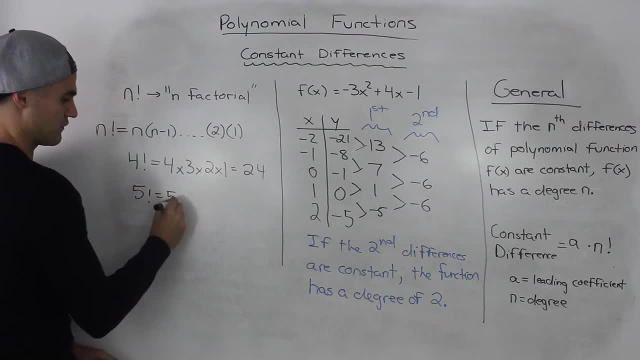 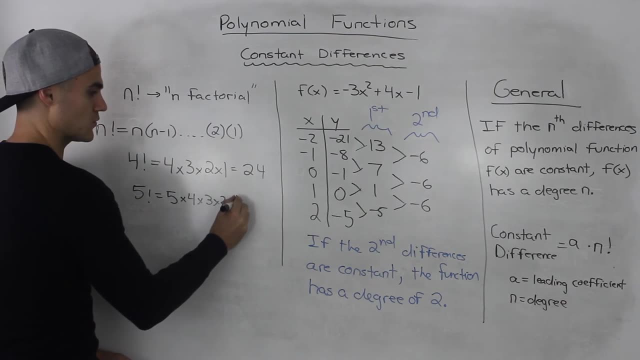 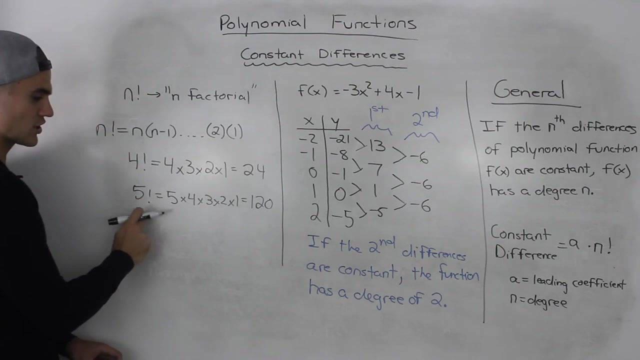 What about 5 factorial? Well, it would be 5, the n value times 4 times 3 times 2 times 1.. So 5 times 4 is 20,, 60 is 120.. You can actually find this on your calculator. 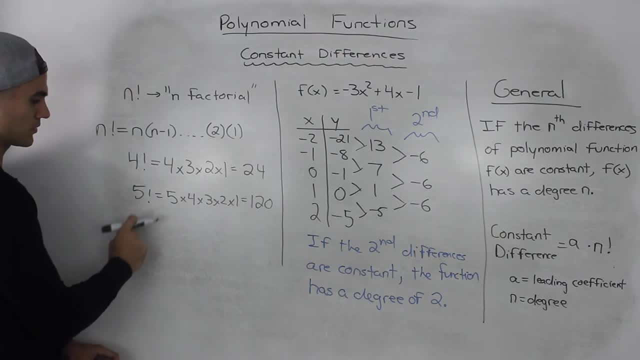 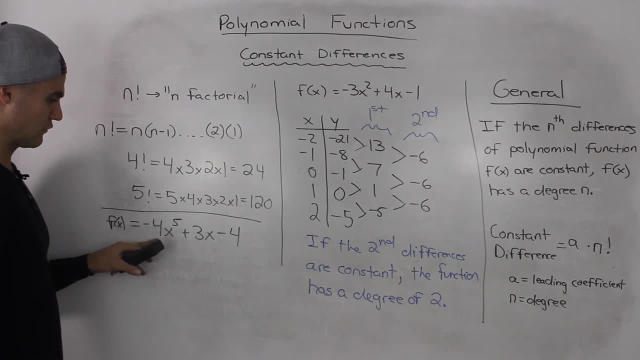 this exclamation mark. So you take a number, put the exclamation mark in the calculator and you should get these values and they're called factorials. So for example, if we're given this function, negative 4x to the 5 plus 3x minus 4, and we 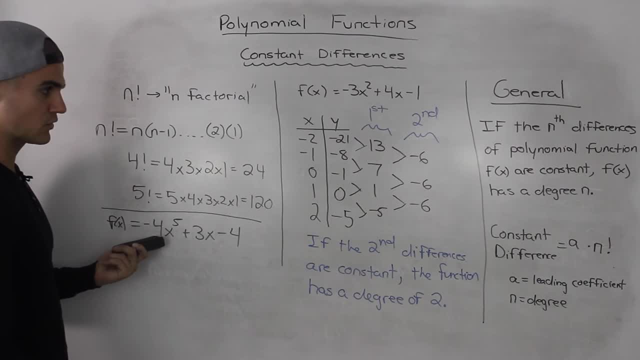 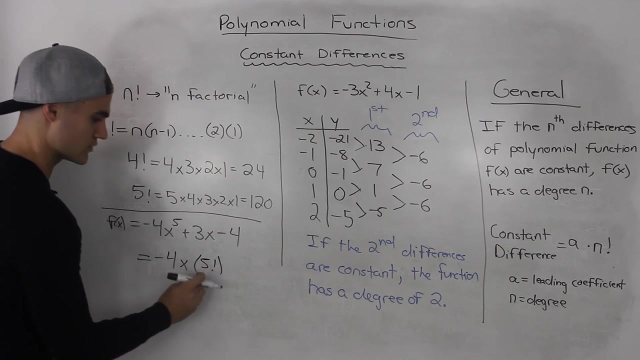 were asked what's its constant difference? Well, because we have the leading coefficient, the a value, and the degree of 5, the n value. we can figure that out. So it would just be the leading coefficient negative 4 times 5 factorial, or the degree factorial, And we 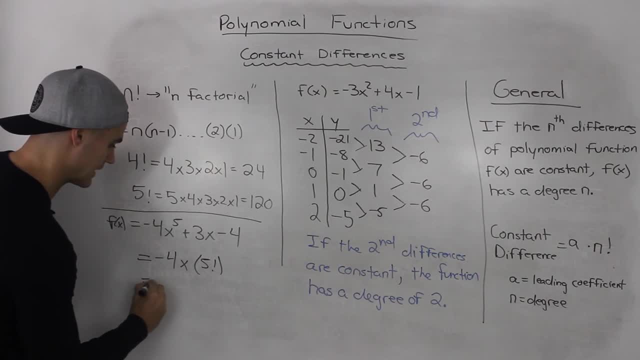 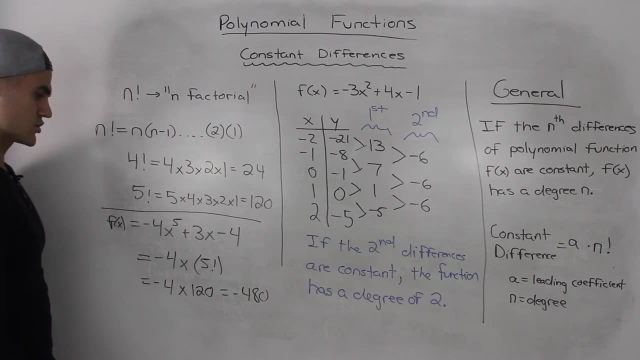 already know that 5 factorial- we did it up here- is 12.. So it would be negative 4 times 120, which would be negative 480.. So if you took this function, made a table of values for it and took the differences, you would notice that. 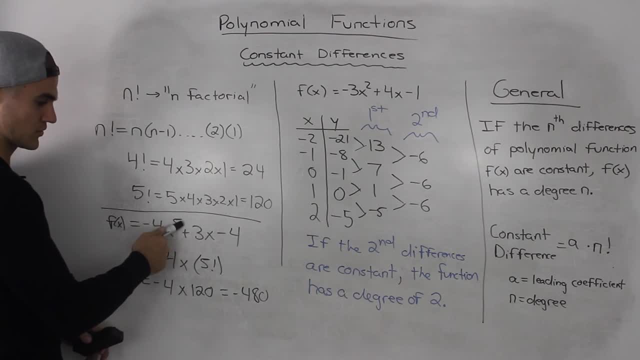